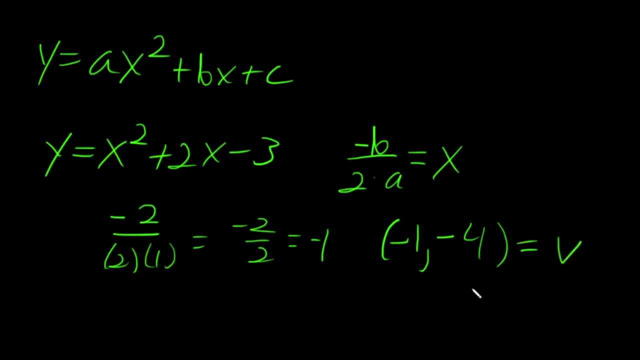 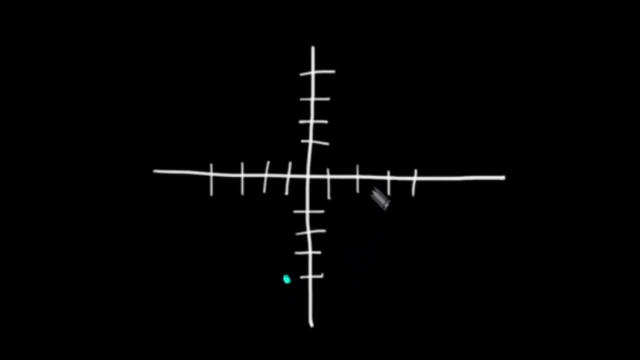 So our vertex is negative 1, negative 4.. So let's plot the vertex: Negative 1, negative 4 is right here And now we need to get at least a couple of other points on either side of the vertex. The first one we might look at is the y-intercept, And that's where x is equal to 0.. 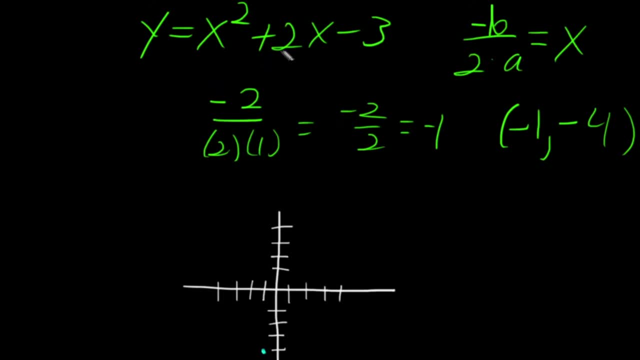 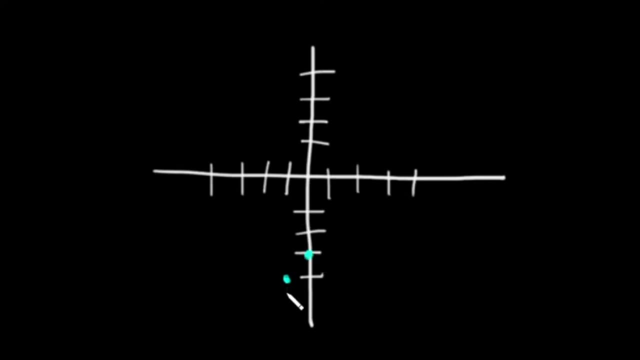 So if we plug 0 back into the original equation, we would get 0 plus 0 minus 3.. And that would give us the point 0, negative 3 right here. Since parabolas are symmetrical about the vertex itself, that means that since we moved over 1, 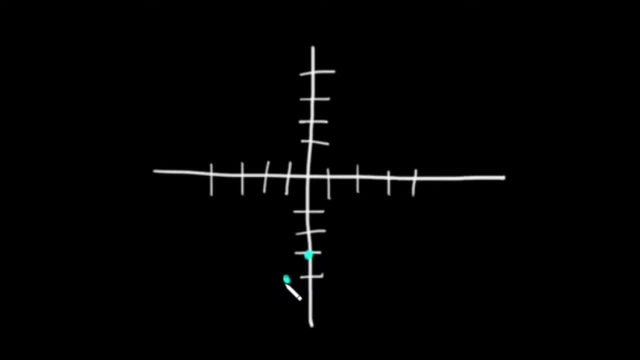 from the vertex to the right and then up 1,. we could do the same thing on the left side. We would move 1 over to the left. That would be negative 2.. And we move up to the negative 3 right here. 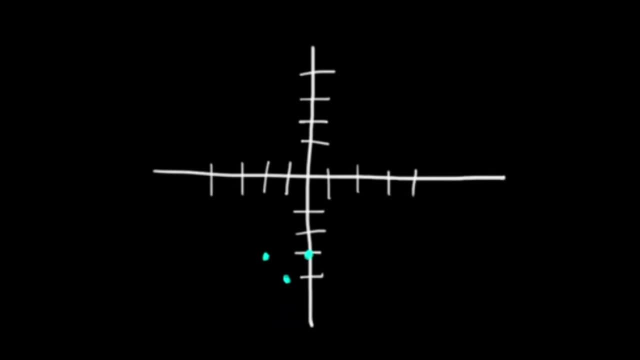 If you're unsure, you could always plug in negative 2 into the original equation and you would get out negative 3.. So we're at the same y-value of negative 3.. 1 to the right went up 1.. 1 to the left also goes up 1.. 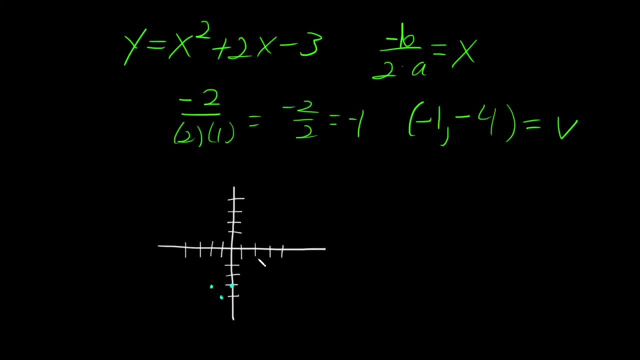 Oftentimes your teacher is going to want you to get not only the y-intercept but also the x-intercepts. The x-intercepts occur when y is equal to 0, which means we can set the original equation equal to 0 and factor. 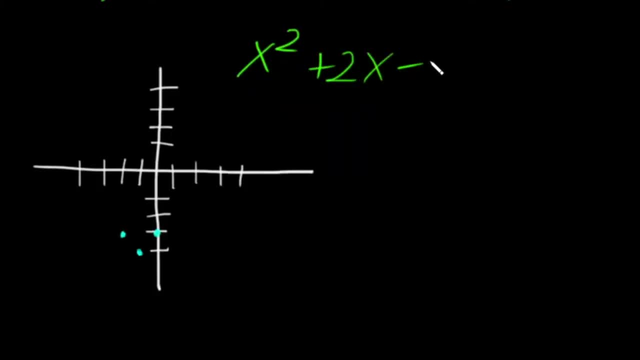 We have: x squared plus 2x minus 3 equals 0.. We need two numbers that multiply to negative 3, but add to a positive 2. Those two numbers would be 3 and negative 1. So our binomials are x plus 3 times x minus 1 equals zero. 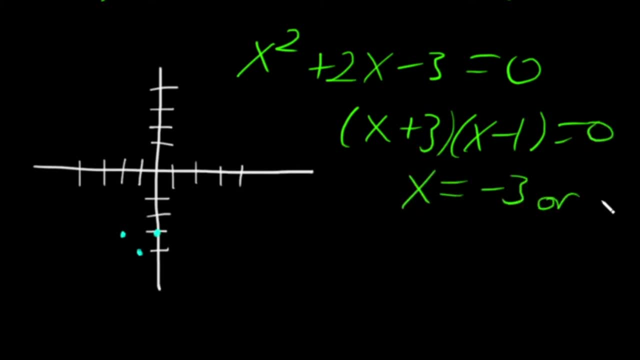 and therefore x is equal to either negative 3 or 1.. At negative 3, we're crossing the x-axis, We're at the edge of our] for x squared, so we have 2x plus 3 times x minus 1 equals 0.處. 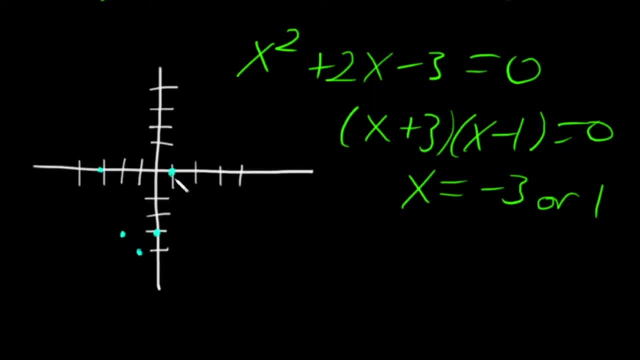 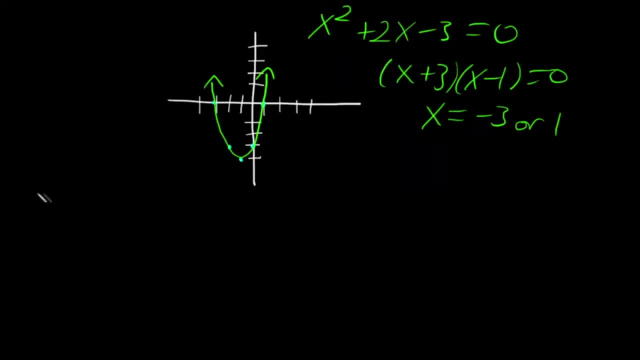 And also at positive 1, we're crossing the x-axis as well And now we can connect the points in a curved manner. We also need to discuss the domain range and axis of symmetry. So the domain, remember, is all of the input values, in this case the x's. 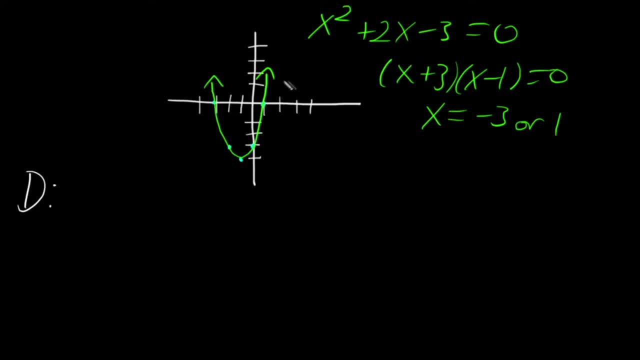 We should be familiar with parabolas that open either up or down, that they spread out to the left and right forever and therefore the domain would be from negative infinity to infinity, which is the same as all real numbers, which could be written like this: 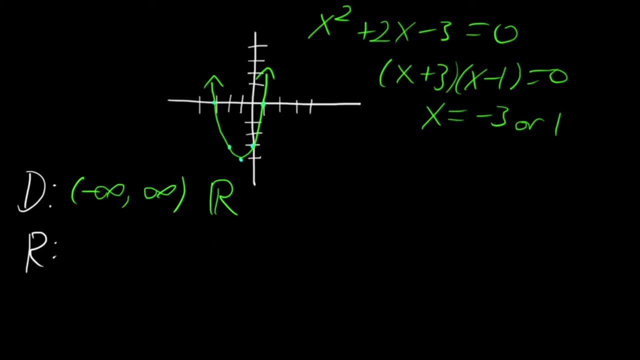 For the range, the lowest value was negative 4.. And since it includes the point negative 4, we're going to use a bracket, and it extends up to infinity. Anytime you're using infinity, that's not included, so therefore we're using a parenthesis. 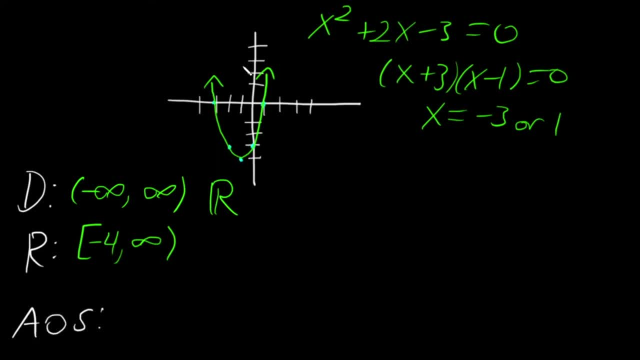 Finally, our axis of symmetry. Remember, that's just the line that splits the parabola in half and it always goes directly through infinity, The vertex, Because it's a vertical line. the formula is always: x equals a number and, in this case, 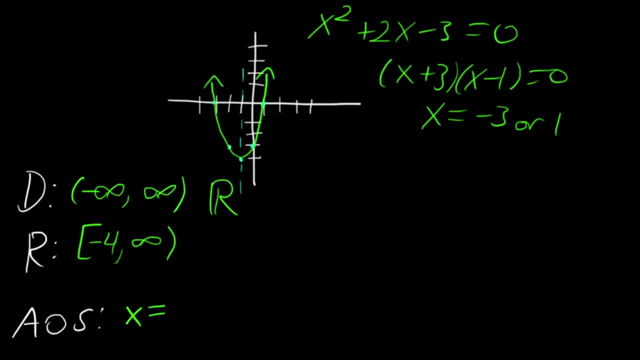 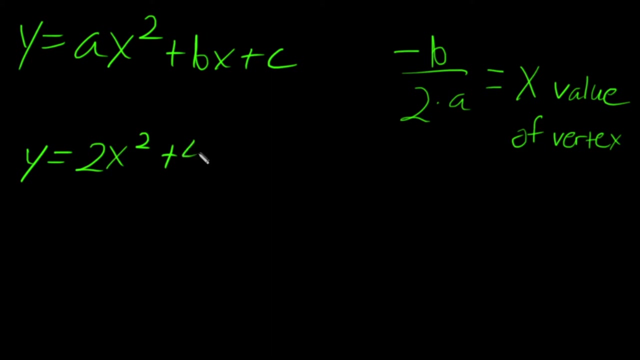 we set it equal to the x-value of our vertex. The x-value of our vertex is negative 1, so therefore, axis of symmetry is x equals negative 1.. Let's try another example. Say we have y equals 2x squared plus 4x minus 1.. 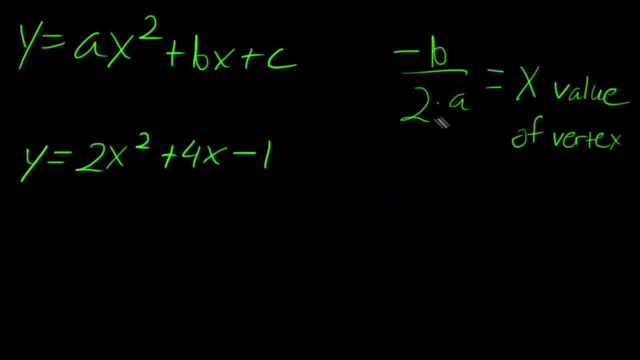 Like before, we'll get the vertex first By calculating the x-value of the vertex Using negative b over 2a. Our b-value is a positive 4, so negative b is negative 4, over 2 times a, which happens. 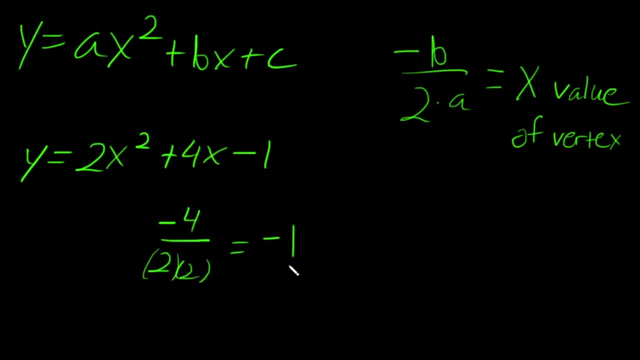 to be 2, and that gives us negative 1.. So our vertex so far is negative 1, comma, and then we'll plug negative 1 into the original equation to get the y-value of the vertex, which ends up being negative 3.. 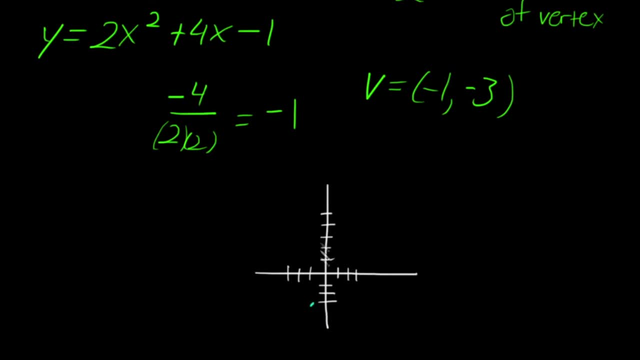 We'll plot the vertex at negative 1, negative 3, right here The y-intercept We can easily get again. that's where x equals 0.. So plugging 0 back in we would get 0 plus 0 minus 1, and therefore our y-intercept will. 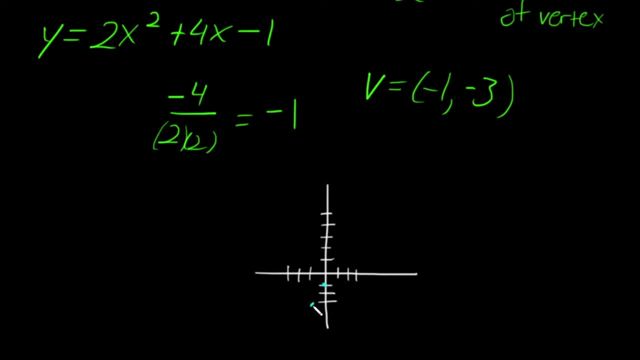 be at 0, negative 1.. In this case we moved 1 to the right and 2 up, So due to the parabola's symmetry, we can go to the left by 1, and still go up 2, giving. 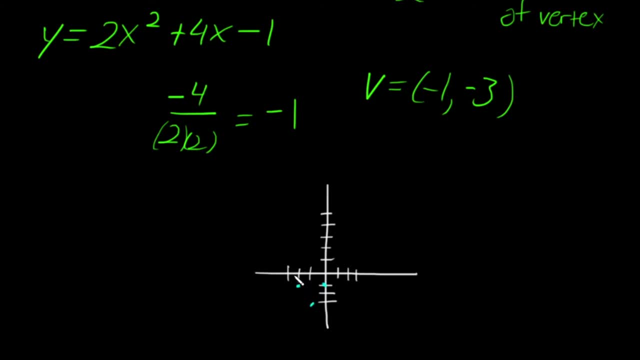 us a second point Now for this quadratic. if you wanted to find the x-intercepts, we could set the original equation equal to 0. And try to factor. In this case it is not factorable. So if you need to find the x-intercepts, you would have to use the quadratic formula. 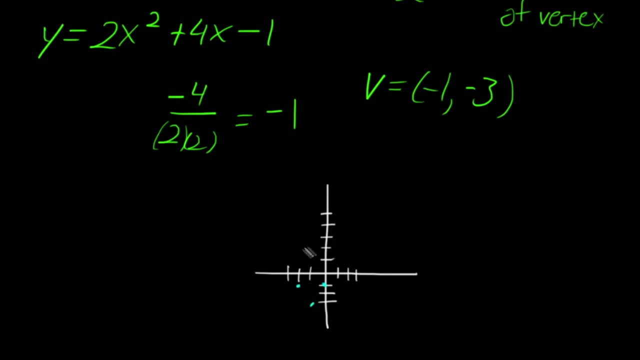 Instead, I'm just going to pick another point to the right and left of our previous points. The x-value at the y-intercept here was 0, so I'm going to pick 1 and plug that back into the equation. If we plug in 1, we'll get out 5.. 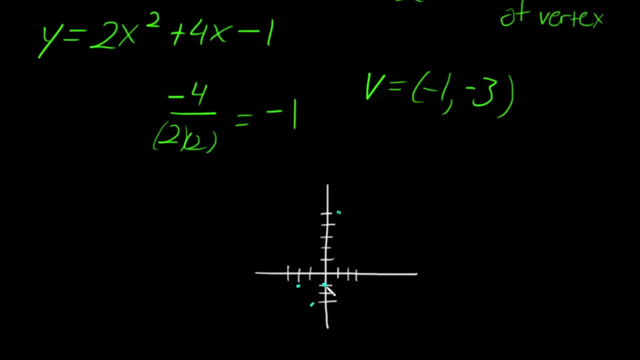 So we're at 1, comma 5.. From our previous point that was a move of 1 to the right and 6 up. so we can mimic that on the other side, 1 to the left and 6 up, giving us the point of negative 3, comma 5.. 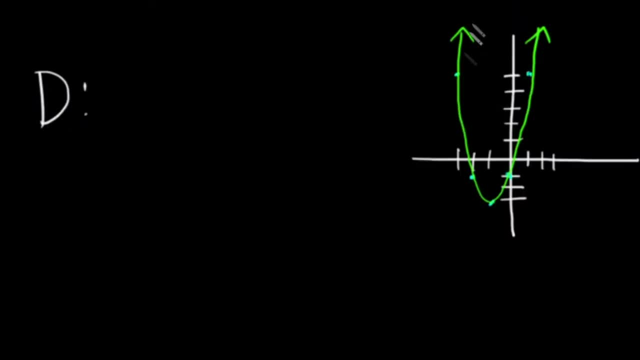 Next we'll find the domain Again. a parabola that opens up or down is going to always spread out to the left and right forever. So our domain is from negative infinity to infinity, or all real numbers For our range. we have a lowest point here at negative 3, and it does include the point 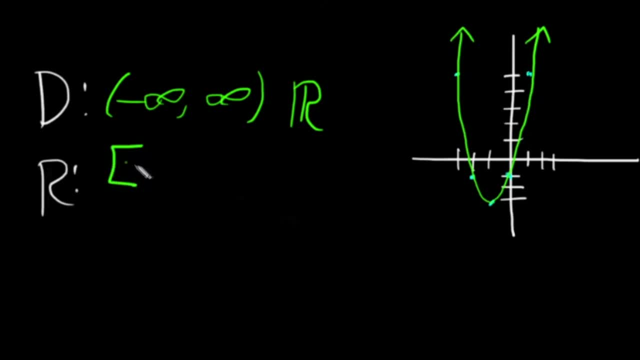 negative 3.. So we'll use a bracket- negative 3, and the graph extends up to infinity. Finally, our axis of symmetry- Again, that's the line that splits the parabola in half- goes directly through the vertex. 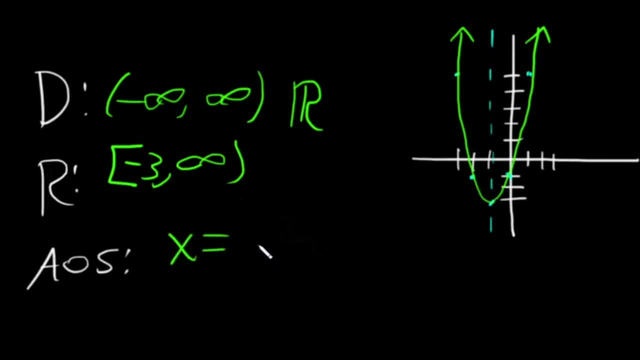 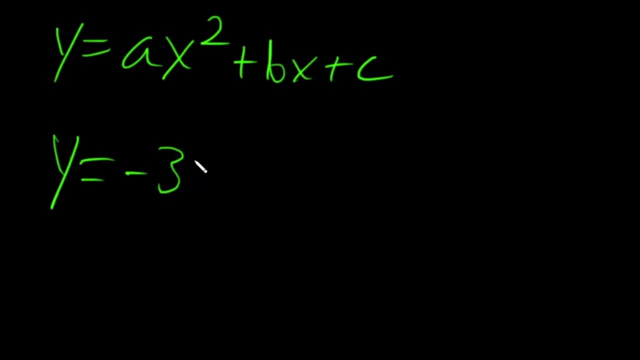 and it'll be: x equals the x-point of the vertex, which was negative 1.. Let's try one more example: y equals negative 3x squared plus 2.. So we'll use a bracket- negative 3, and the graph extends up to infinity. 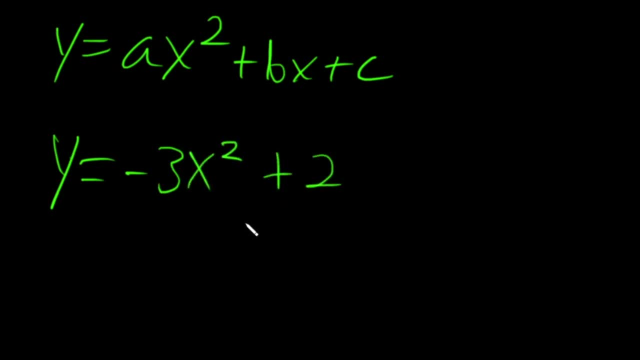 Finally, our axis of symmetry- Again, that's the line that splits the parabola in half- goes directly through the vertex and it does include the point negative 3x squared plus 2.. Hopefully you noticed that there is no b term. 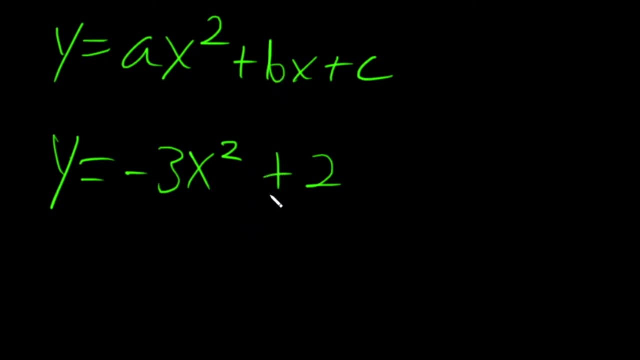 In fact it is a 0. There could be a 0x in the middle here. So when we do negative b over 2a, that's simply going to be 0 over 2 times the a value negative 3.. 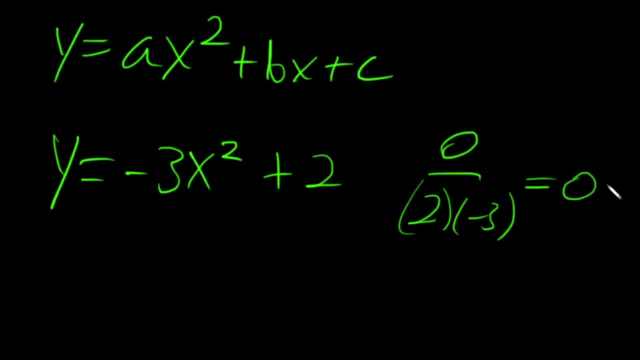 And of course, 0 divided by negative 6 is going to be 0. So far our vertex is 0, comma and we'll plug 0 back into the equation and get 2.. So our vertex is at 0, comma 2.. 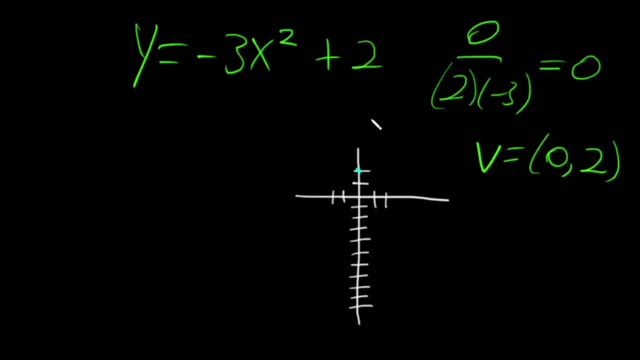 Our vertex is right here. That's also the y-intercept, so we don't need to solve for that. But like the previous example, we would need the quadratic formula in order to solve the x-intercepts. So instead we'll just find a couple of points to the right and left of the vertex. 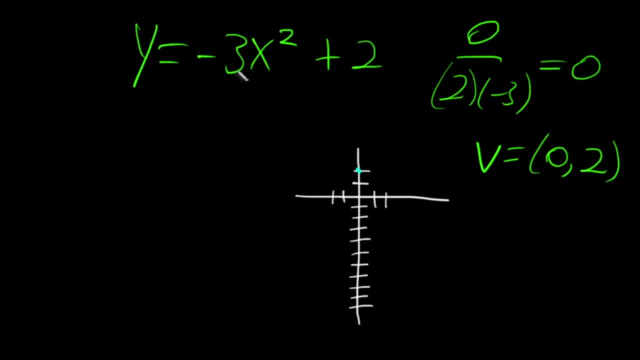 So if we go 1 to the right, that's an x value of 1.. And if we plug that in, we'll get out negative 1.. So our point is here, And therefore, by moving 1 to the left, we'll also be going down to negative 1..